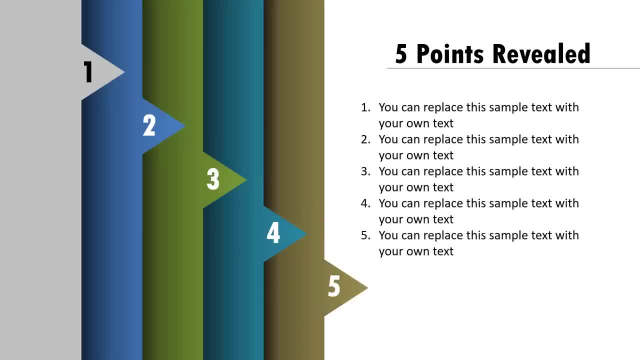 The third point, the fourth point and the fifth point. Now, if I want to go further into any of the points, I can click on the specific number. For example, if I want to talk further about point number 3, I can click on the number and that will take me to slide number three. 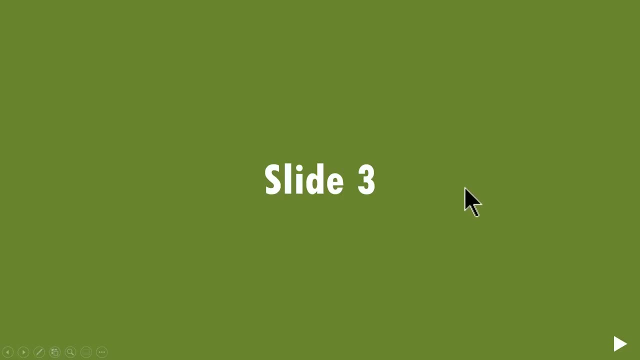 Here I can give all the details I want. Once I finished explaining my slide three, then I can previously Click on 3.. Then I can click on preview at the top of the page and I will see that I have my pre scenery header. 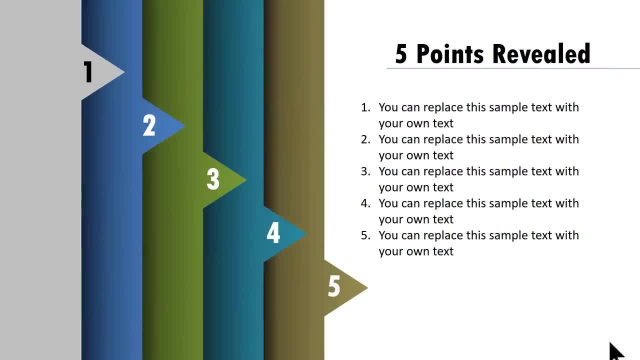 Here. if I say I want to specify which points, Then I will look at the information that may be there. by placing so many points and, for example, the audience, I can click on this small white arrow here and that will take me to the dashboard slide. 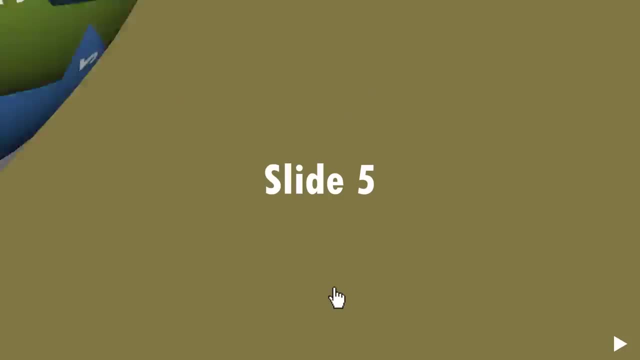 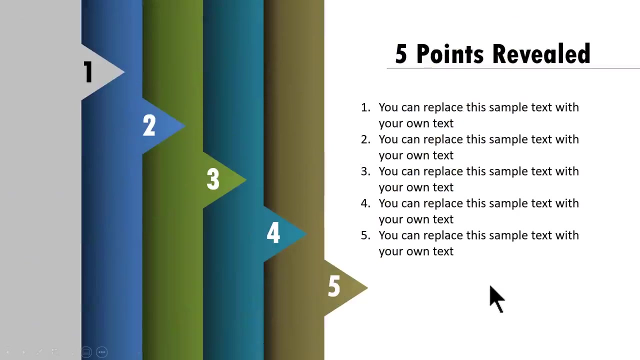 And if you want to talk further about point number 5, I can click on that point and that will take me to slide 5 and I can give all the details. and I can come back to the dashboard slide by clicking on the white triangle. 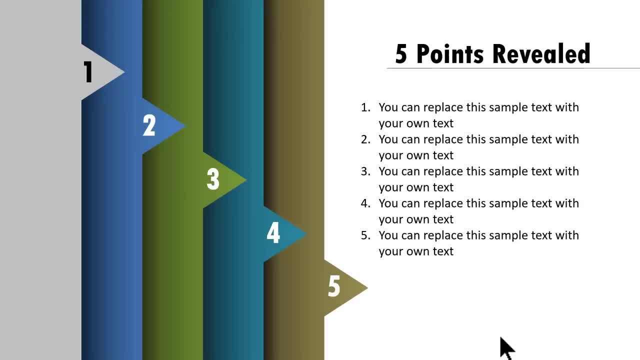 So this is the basic setup. You can extend the same basic idea to create any kind of interactive slide deck. By the way, we created this interactive slide deck by using links in PowerPoint. Let me show you how to create this beautiful slide deck from scratch. 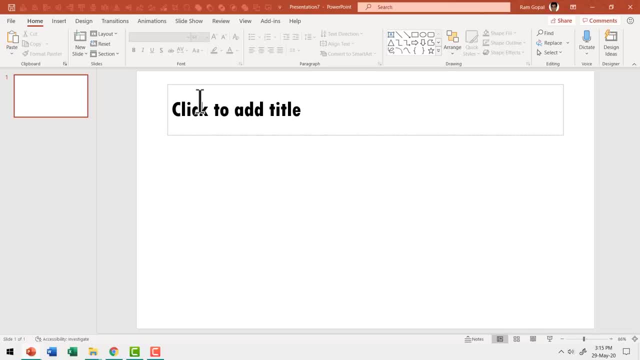 Here I have a new presentation and I'm going to start my presentation by writing my slide title here. Let us say 5 points, and I'm going to have this right aligned by clicking on this option here. Then I'm going to create 5 bands that will help me to introduce the overview of 5 points. 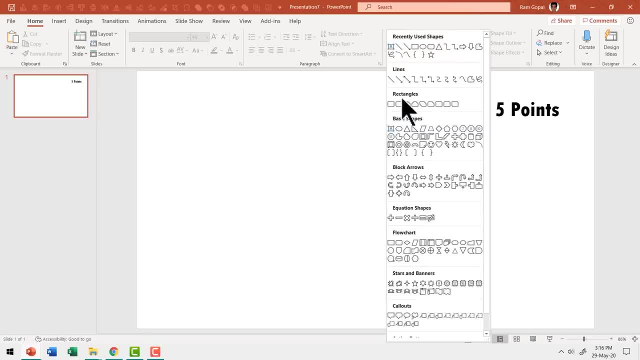 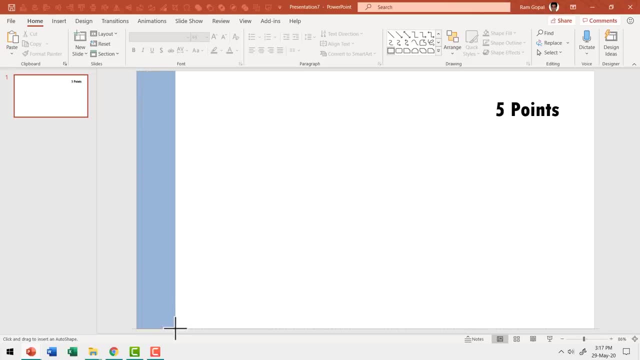 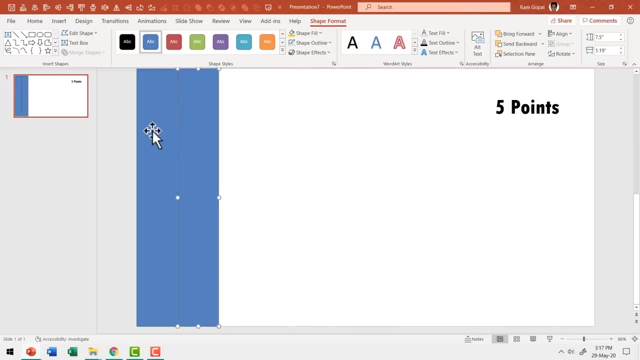 To create the bands, I'm going to use a simple rectangle tool. Let me go to rectangles in AutoShape's gallery, Pick up the rectangle tool And let me draw a small thin, narrow, rectangular band like this. Now let me press Ctrl D and then place a copy of this right next to the previous strip. 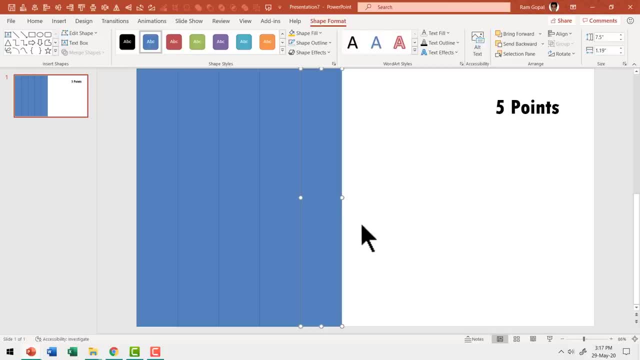 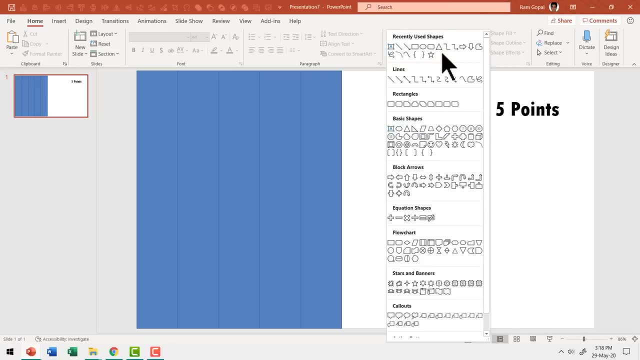 And then let us press Ctrl D again, again and again. The next step is to create a handle for each of these bars, which will serve as number placeholder. So let me go to AutoShape's gallery. From basic shapes, let us pick up this isosceles triangle, hold the shift button down as we 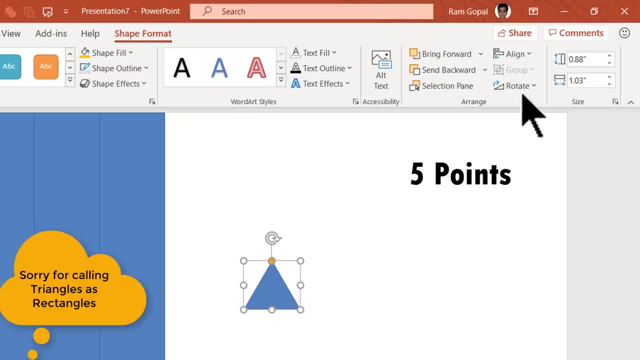 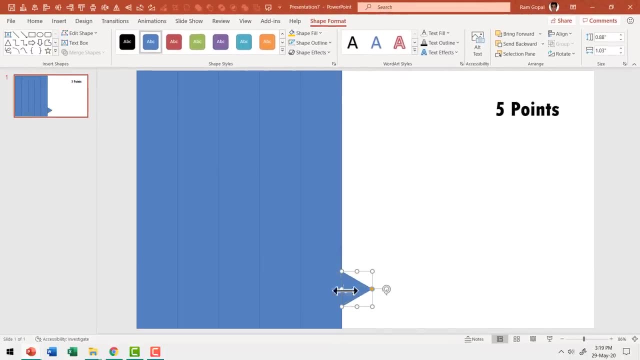 draw a rectangle like this, And then let us go to rotate and then say: rotate right 90 degrees, and then place this somewhere over here And it has to touch the bar like so, And then I'm going to make 4 more copies. 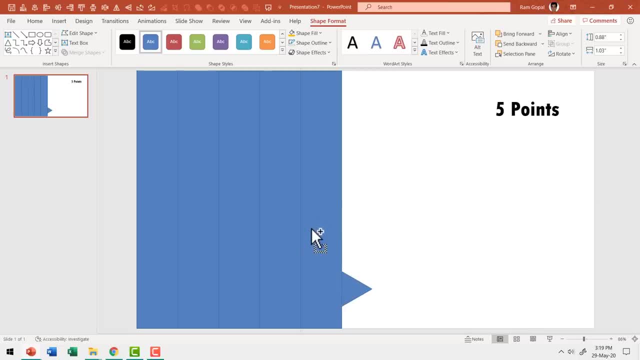 So I'm going to hold the control button down as I place the next one right above this, and then above this, above this. Don't really bother too much about the position right now. All we are bothered about is to have 4 of these rectangles. 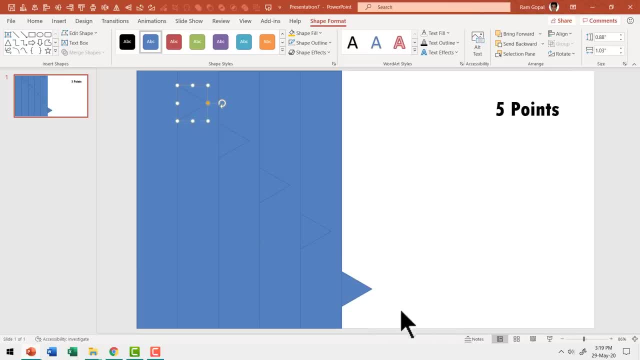 The next thing I'm going to do is to ensure that there is equal distribution of space between these rectangles. So I'm going to click and drag my cursor across to select all these 5 rectangles And then let me go to shape format, go to align and say: distribute, distribute vertically. 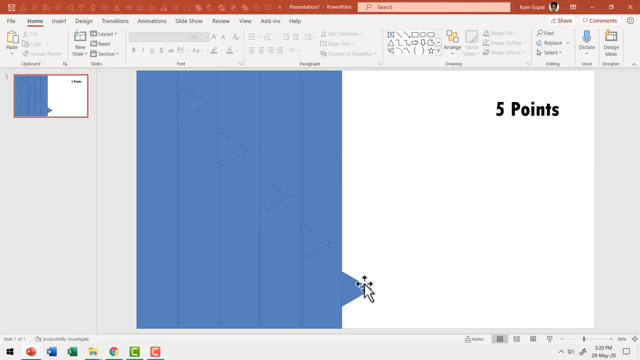 Now this looks perfect. The next step is to merge the bar with the handle, So I'm going to select the first one. hold the shift button down and then select the rectangle, and then go to shape format, merge shapes and then say shape union. 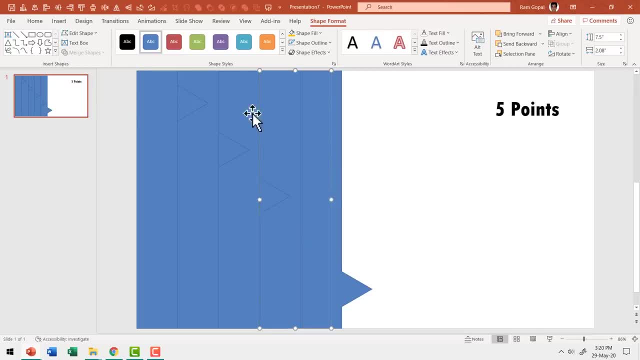 We do the same thing for the next one as well: Merge shapes- shape union. Next, I'm going to use the text box tool to write a number on the handle. So let me go to the text box tool in Autoshapes gallery, write number 5, because we are going. 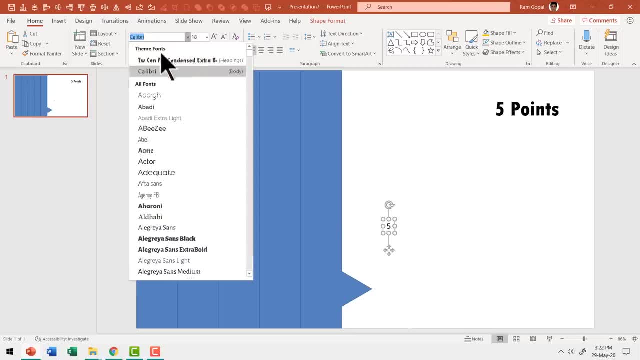 to have 5 points, and then let us make it really thick and bold. Let us use Toussaint- empty, condensed- extra bold. You can use any other font which is your favorite, and I'm going to place this right above here and that looks good. 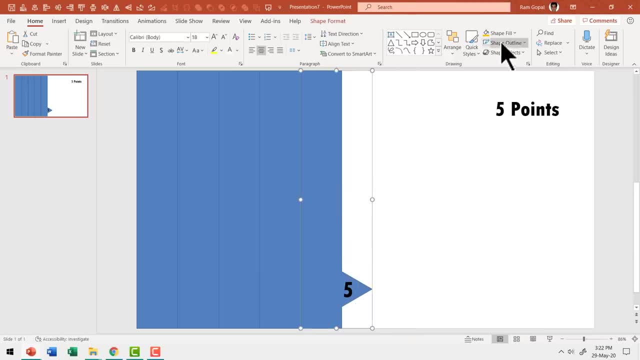 Now I'm going to give this a distinct color. Let us choose one of the fill colors, like, say, this orange color, and then I'm going to give this gradient. So let us go to shape fill, go to gradient, and I'm going to use this gradient here, called 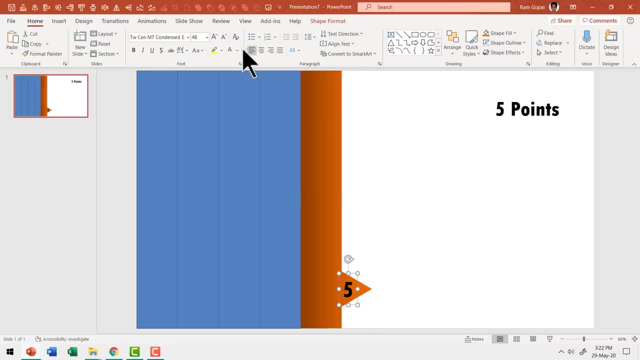 linear. right Now, let us give this number white font color. Let us go here and choose white font and then let us select the number and the shape behind it and press control G, which is a shortcut for group, and I'm going to place this right. 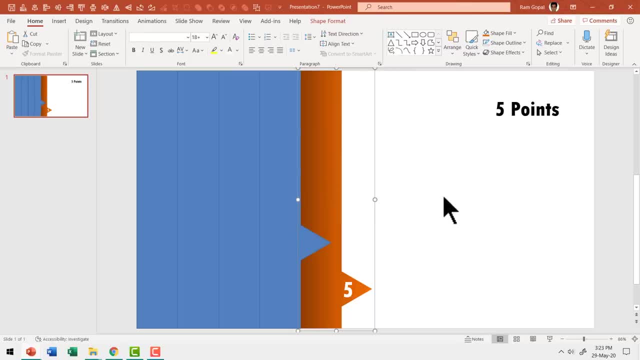 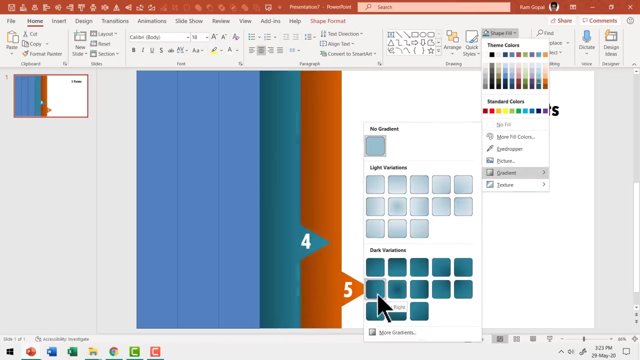 behind. So I'm going to right click on this And we're going toů Change the font colour to white so that we will be able to operate C code group and stay even. We're going to select the gradient from these colors, ensuring that we do not need it in. 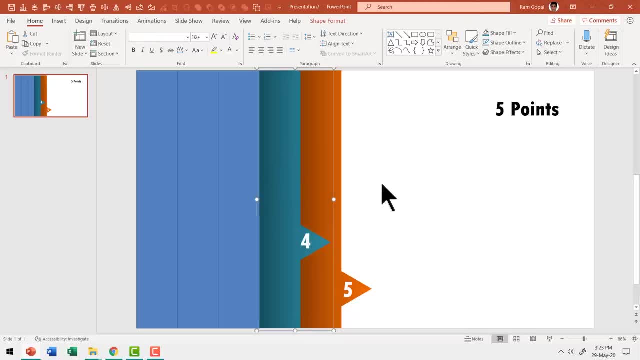 the regular chat And I'm going to change the color to black. So I'm going to onions. I want to add one, the new compose text, document, text, document, text. and I'm going to Druckstrap this and I'm going to work it and I'm going to press control. 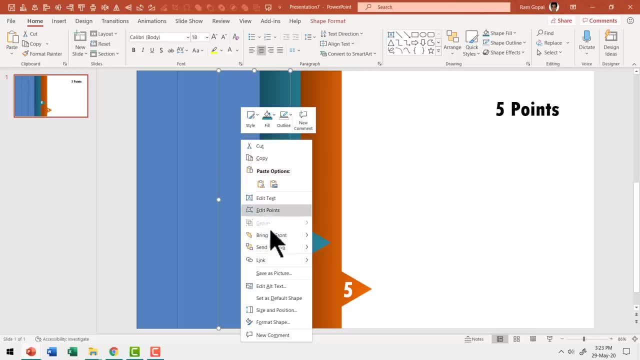 G to group it, the next one forward by right clicking and using the bring to front option. Once again, I'm going to select the same number- placeholder, press, control C, control V- and then place this over here, and then I'm going to replace this with number 3 and then let. 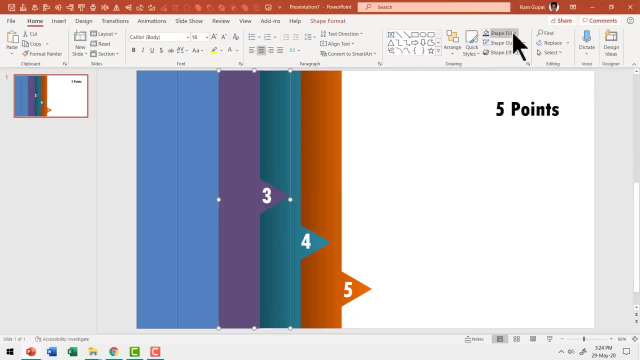 us choose a different color for this, maybe this kind of purple color, and use the same gradient, linear right, and then do the group Once again. let us bring this forward. Finally, for good order sake, let us select all the shapes and ensure that there is no 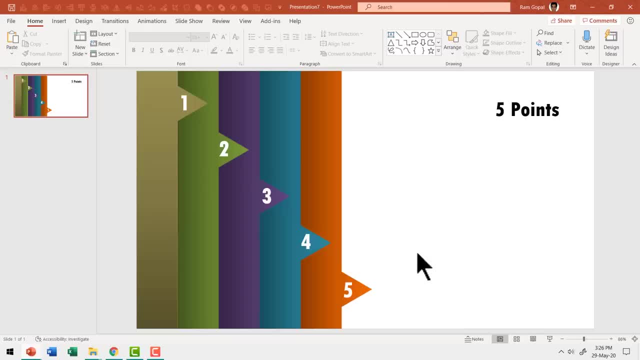 outline whatsoever, and this is how the final shapes look. Now let us write the text for five points. that will lead to five different slides. We can use either the text box tool or we can always change the layout to title and content and we can write our text. 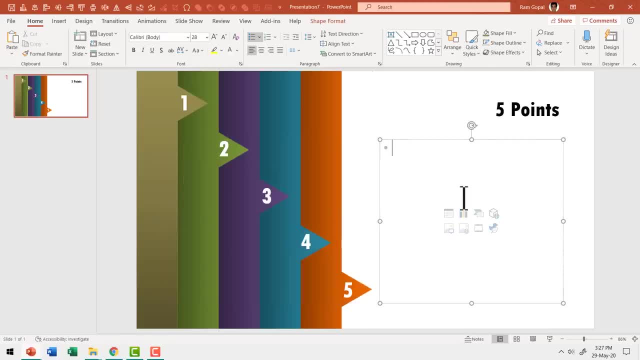 So let us readjust the size, like so, And then let us have the first point, and then you can continue doing so for the remaining four as well. Now it is time to add some animation to bring excitement to this slide. Let us select each of these groups. select the first one. hold the shift button down. 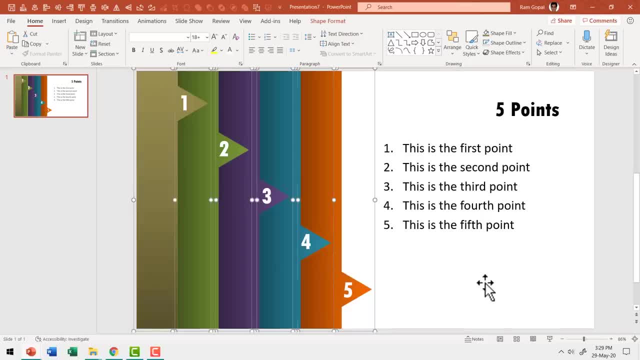 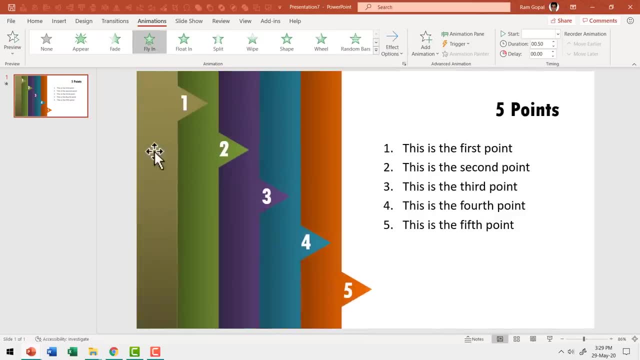 select the second one, third one, fourth one and fifth one and then go to animations and say: fly in animation, and it is to happen from left. So that is how the animations happen. Then we need to have these animated as well. So I'm going to select all of this text and then let us add a simple fade animation and 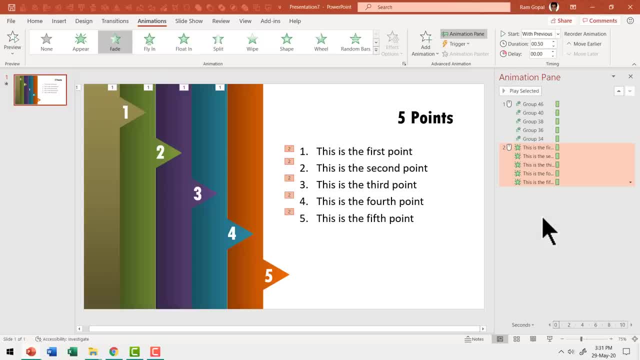 let us go to the animation pane and see how the various animation events are shown. First, we need to have each of these numbers come on click. So we need to have the first five animations happen on click alone. So let us have start on click for the first five events, and these animations need to happen. 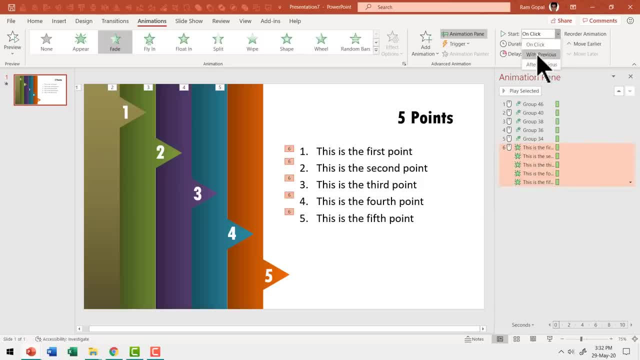 with previous. So I'm going to select all these And then say: with previous. Now all that is left for us to do is to ensure that this animation matches the arrival of this one. So I'm going to have the first point, move to the arrival of this group and then the 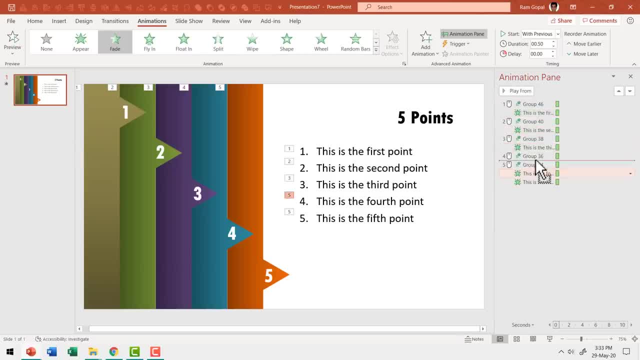 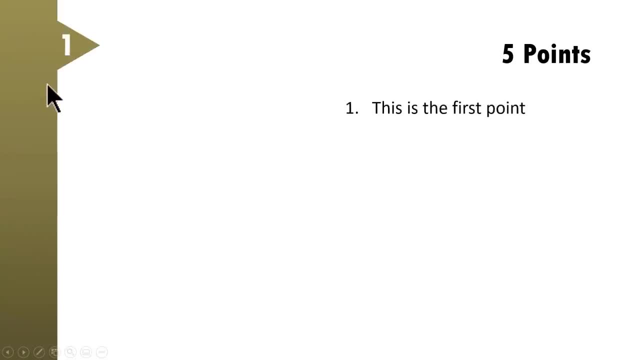 second, one to the second one, third to the third, fourth to the fourth and the fifth one. So the way the animation plays is: on a click you can see we have the first group enter and we have the first point shown and then the second group enter, the second point, the. 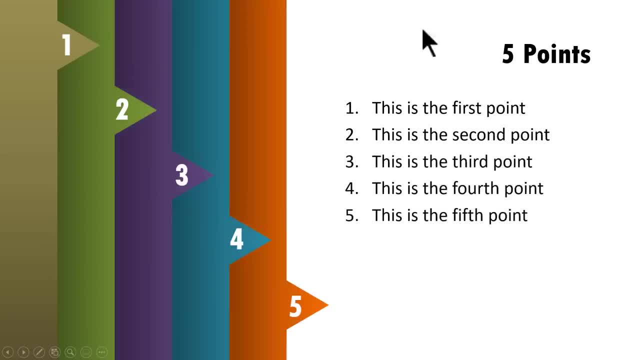 third group, The fourth group and the fifth group. Now we've got our basic setup slide ready. Now we need to link each of these to the corresponding slides, and that is very easy. Now let us add our first slide here by right clicking and saying new slide, and let us call. 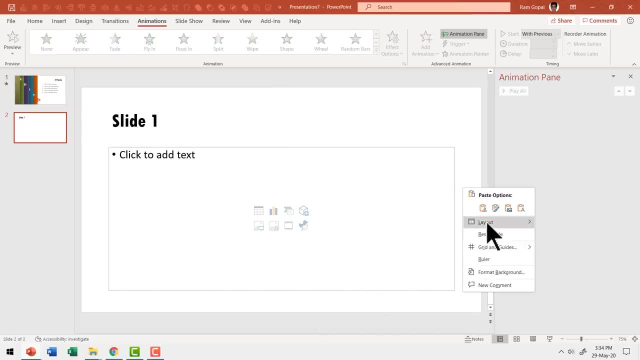 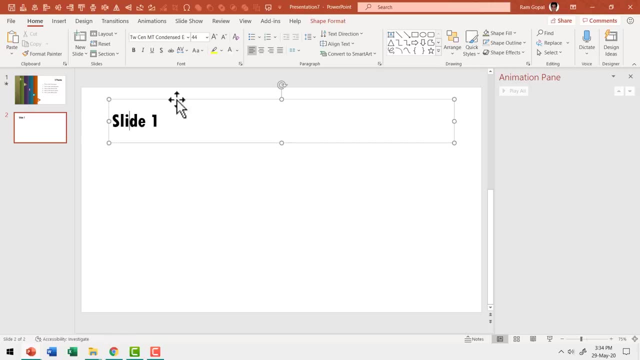 this slide one and let us have the layout as just the title only layout. Now I'm going to have this right in the center and middle, So let us select this and have this centrally aligned and then go to arrange, align and say align middle. 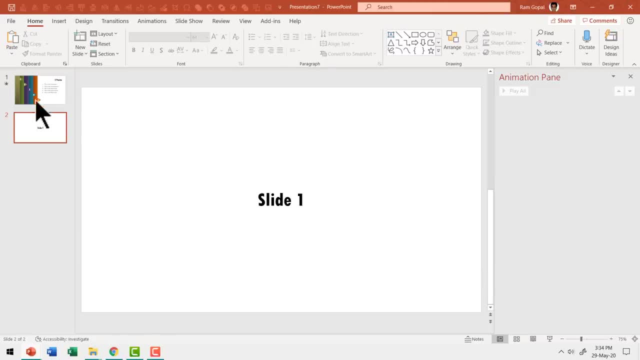 Now I'm going to give this slide a certain color and that color is going to match the color that we see here. So the first color is the golden color. So I'm going to right click, go to format background and say solid fill for the background. 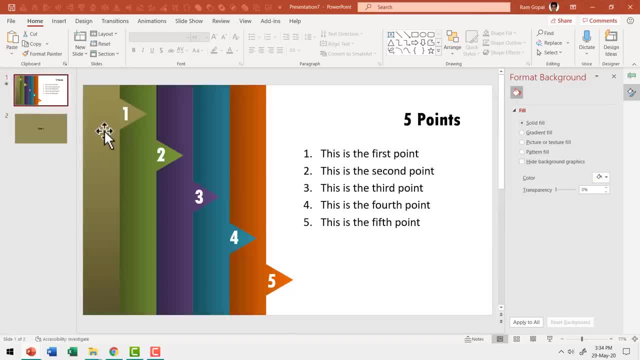 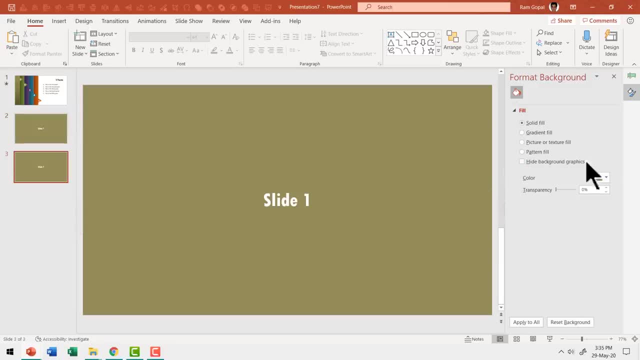 and let us choose this color, because this is the color that matches number one, and let us change the font color to white and let us duplicate this slide and the format background for the second one is green, So let us select that and then change this to slide two. 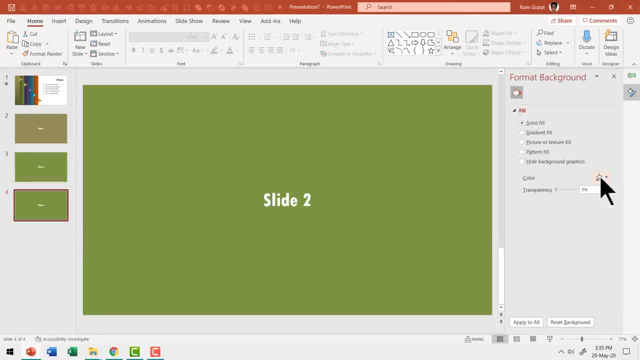 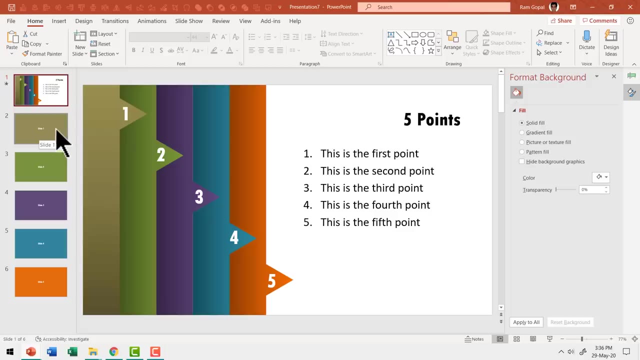 Let us duplicate this slide. The next one, the background is purple. We are going to call this slide three. Now we have got five slides. Now we need to link each of these numbers to the corresponding slides. Let me select number one here. 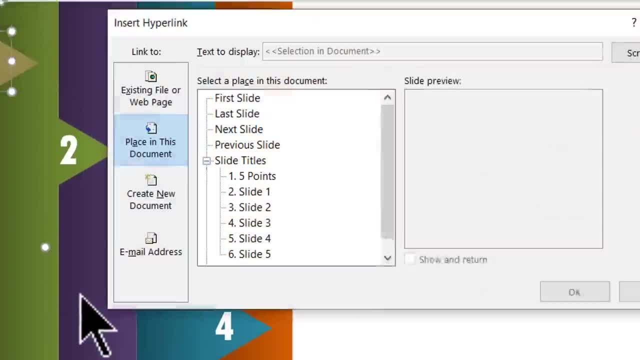 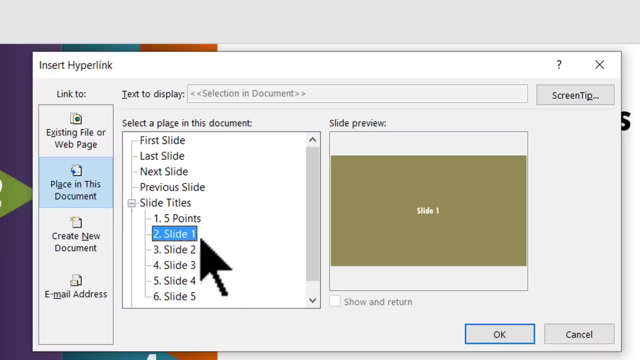 Right click on number one and then say link and that will take you to this dialog box. Go to place in this document and then click on slide one And you can see a preview of that slide And if you think that is the right one, you say okay. 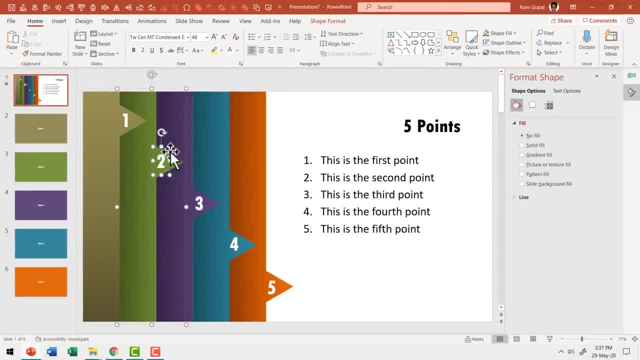 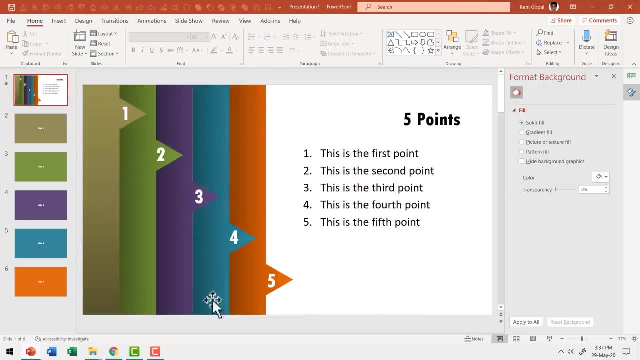 Now this number is linked to slide one. Right click on number two and then go to link and say slide two and say, okay, We have now linked each of these to the individual slides. We also need to find a way to link each of these slides back to the main slide. 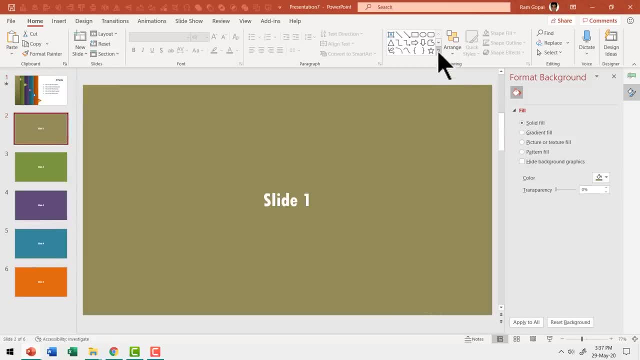 So Let us go back to slide one here. Let me create a small triangle that will take me to the first slide. Let us go to basic shapes: isosceles triangle. hold the shift button down As you draw the triangle. go to shape fill: white fill shape outline: no outline. 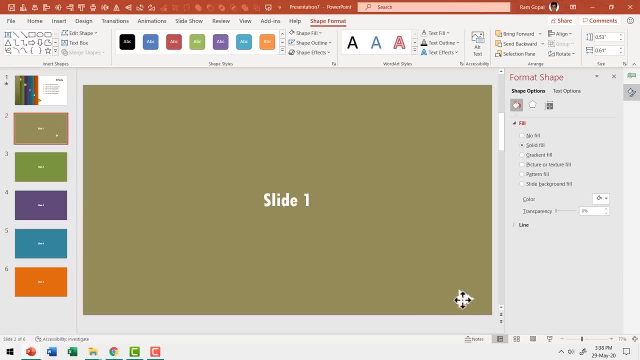 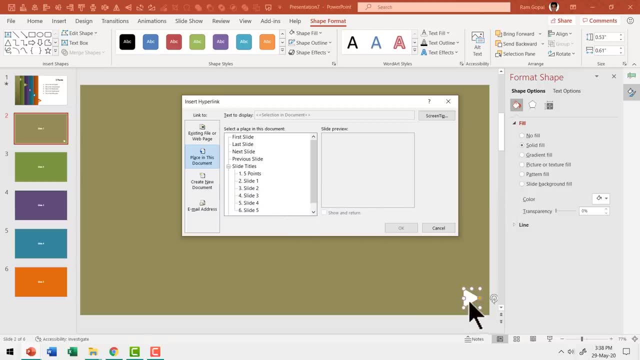 Then go to rotate, rotate right, 90 degrees and place the summer over here, And then right click on this object, go to link, And this time you link this shape to the first slide, which is called five points, And you say okay. 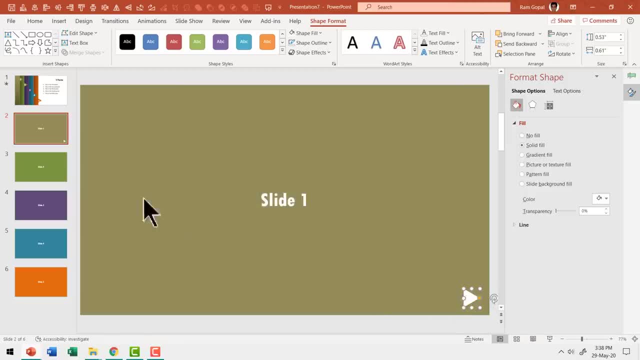 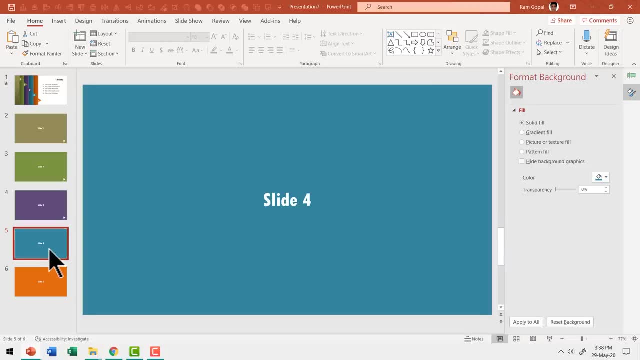 Now you make a copy of this by pressing control C and then go to each of the slides which you want to go back to the first one and then paste it by using control V option. Now we've got, for each of the slides, a connector to the first slide. 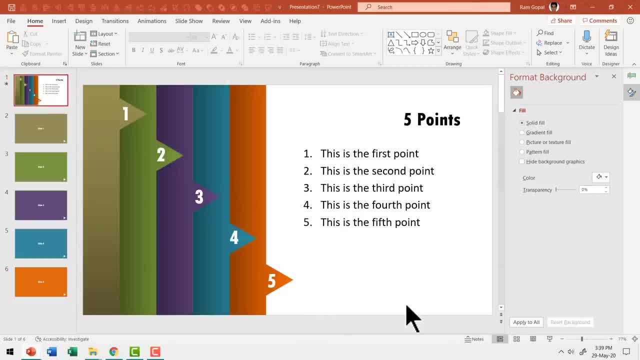 And the first slide is linked to five other slides. And finally, to add a little bit of drama, I'm going to add transitions to all the slides. So I'm going to select all six slides while holding the shift button And then I'm going to go to transitions and I'm going to use a simple peel off transition. 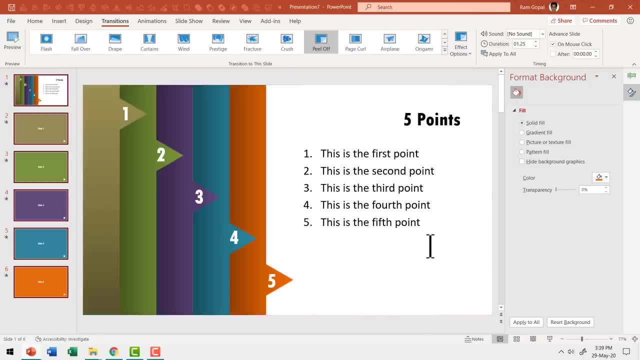 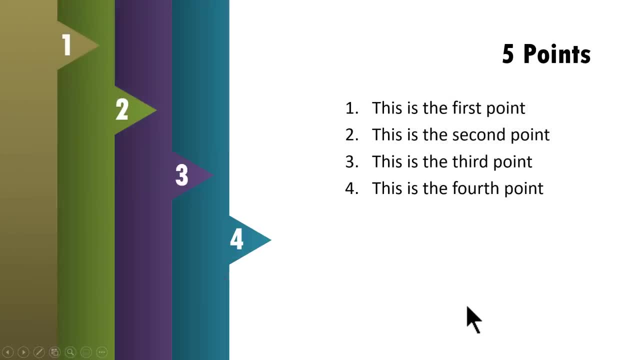 in the exciting option, And this is how the transition plays. Now let us go to the first slide. I bring in each of these points and then I give an overview of the five points here And then, based on the request from my participants, I can go to any slide I want. 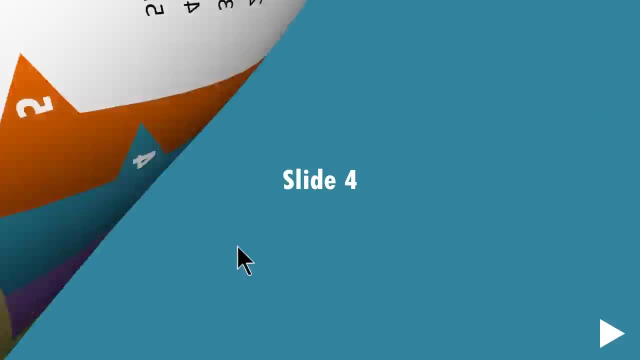 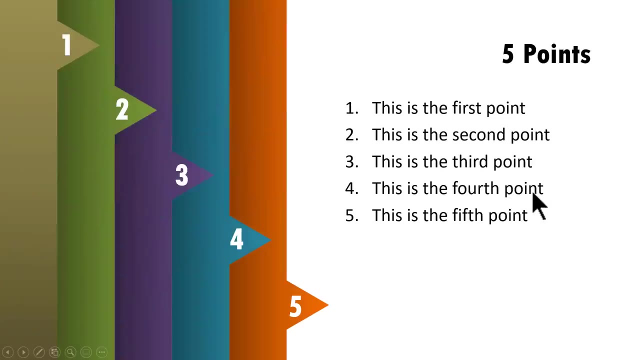 For example, if I want to expand on point number four, I can click on that, and that will take me to slide number four. I can click on this. I can click on the white triangle, and that will take me to the first slide. 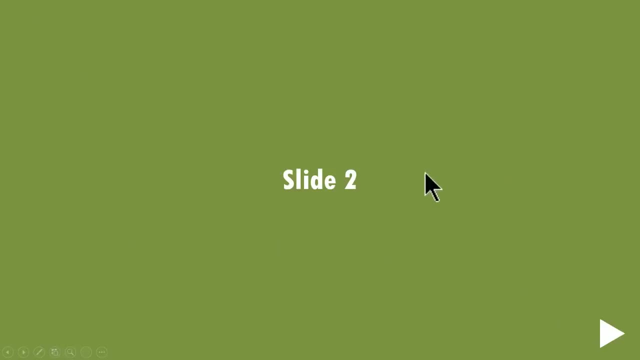 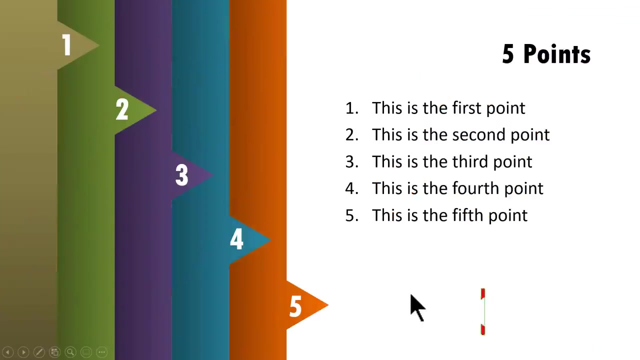 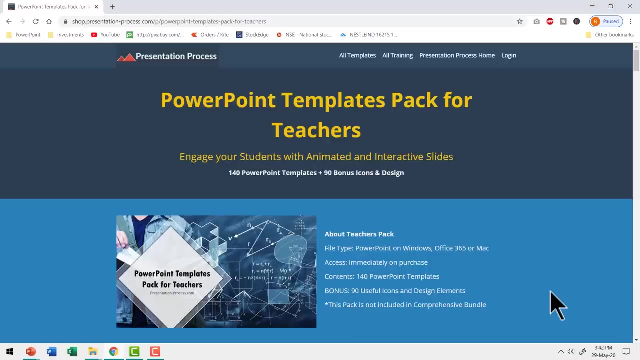 And then let us go to point number two, expansion. And this explains point number two, And then let us go back here and point number five and then go back here. So that is how we create an interactive slide deck. We created this tutorial especially for teachers, because there is a lot of requests from teachers.